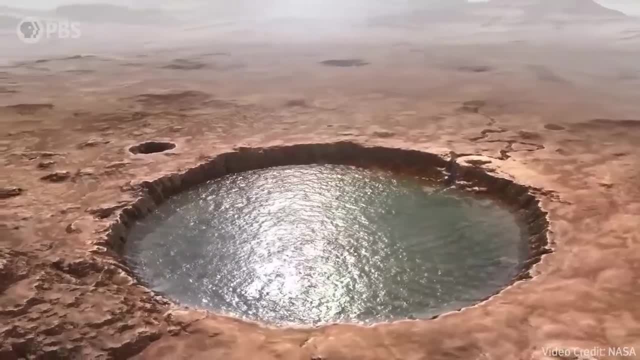 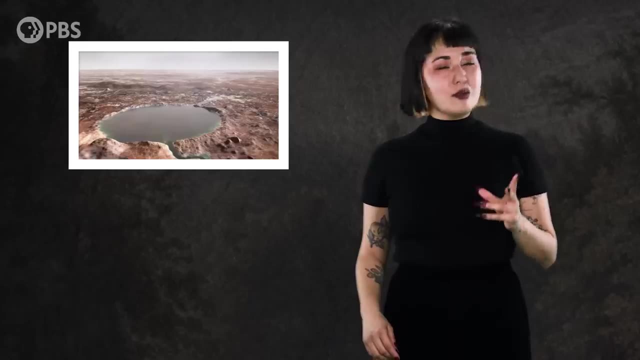 Floods like this were fairly common on ancient Earth. But this was not Earth. This was Mars. But at a time in the deep past when it was much more… Earth-like. 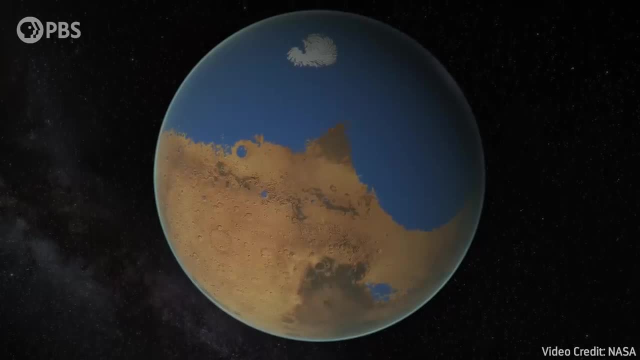 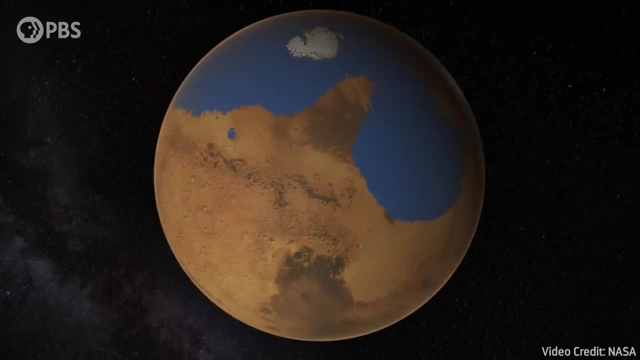 It had big bodies of liquid water on its surface. It had a protective and insulating atmosphere. It had a warmer climate. And maybe, just maybe, it had life. 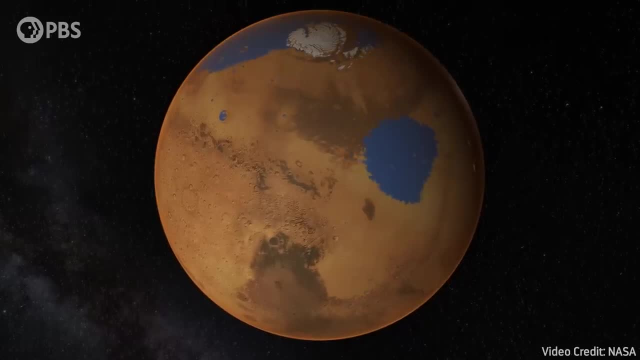 As far as we can tell, though, it doesn't have any of those things anymore. Here on Eons, we're going to talk about some of the things that have happened in the past. 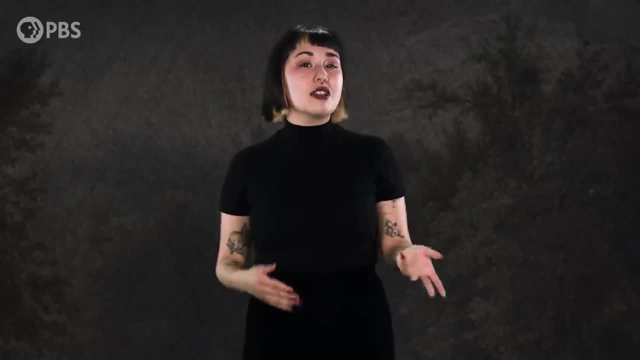 Here on Eons, we're going to talk about some of the things that have happened in the past. For instance, we often talk about the radical changes and countless revolutions that our planet has gone through over deep time. 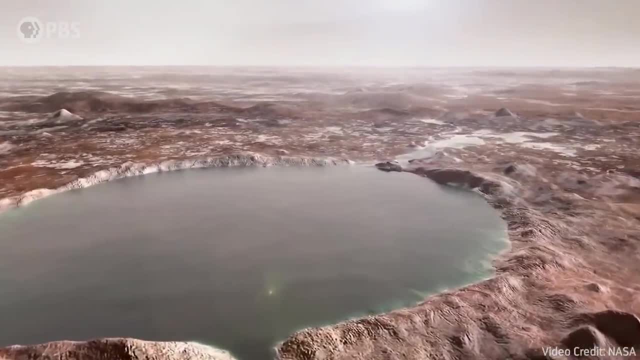 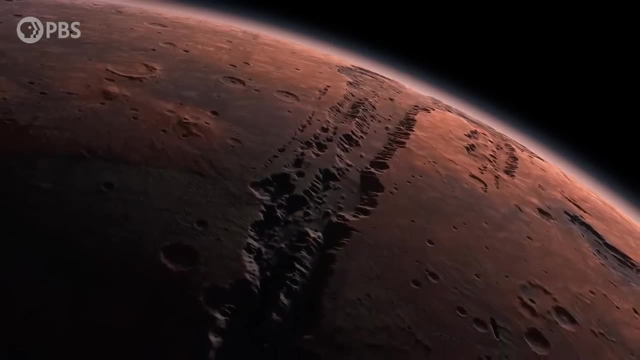 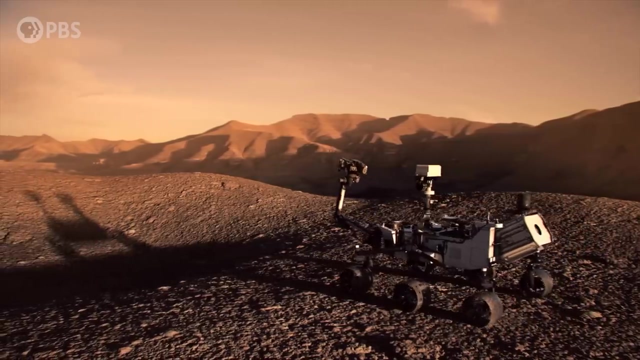 But while Earth's natural history has been playing out over the last few billion years, another epic planetary saga has been unfolding right next door. Even though we've been asking questions of that red dot in the night sky for a long time, we've only just recently begun to figure out some answers, thanks in large part to our curiosity and perseverance. 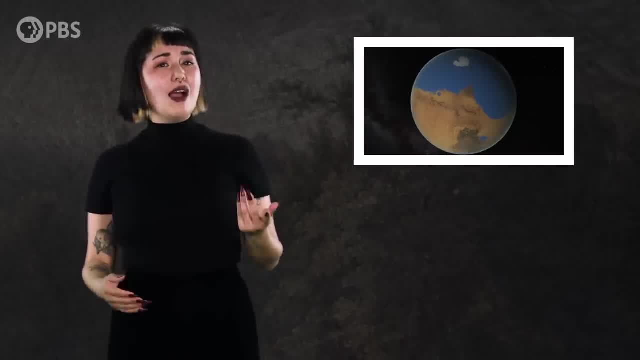 So what happened on Mars? How and why did it go from that warm, wet, potentially habitable planet to the cold, dry, inhospitable one that we know today? 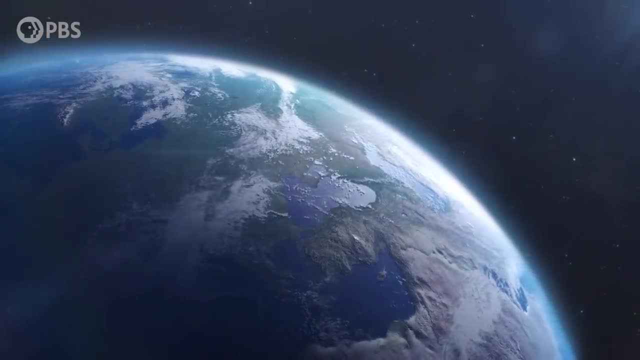 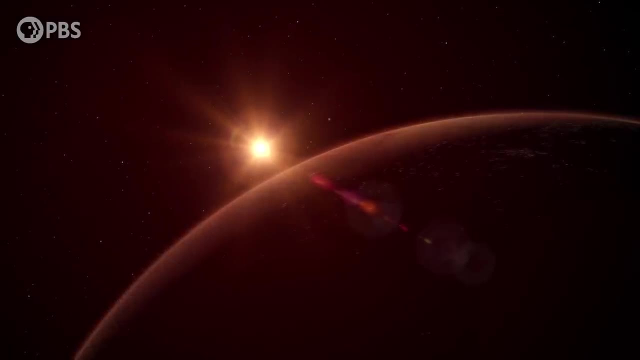 Well, the core reason seems to be that while we had some surface-level similarities at one point, internally, our two worlds were on very different trajectories. 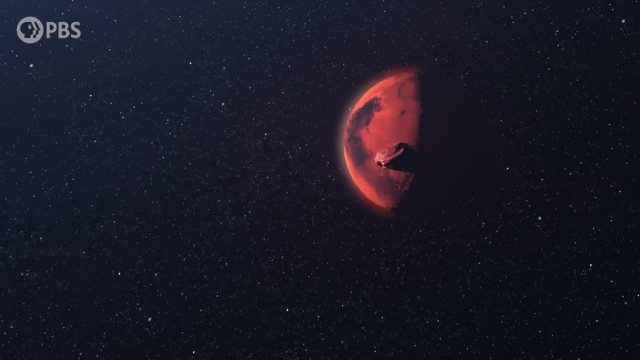 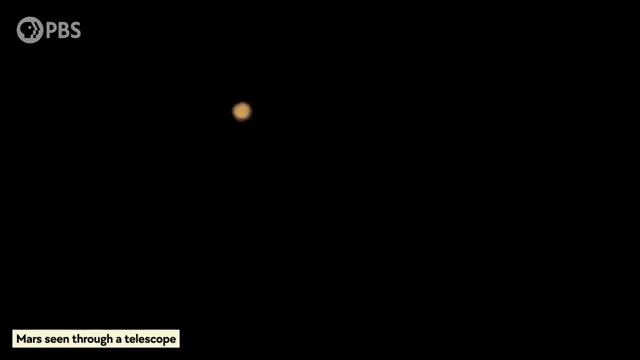 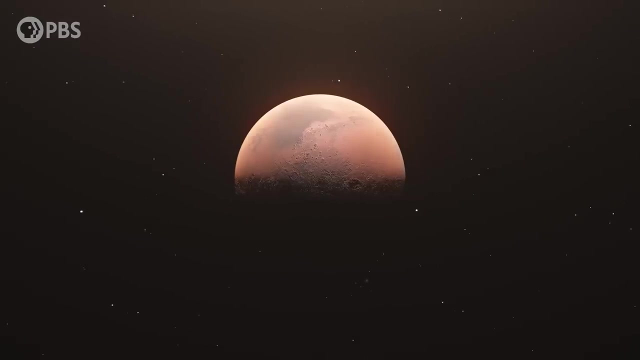 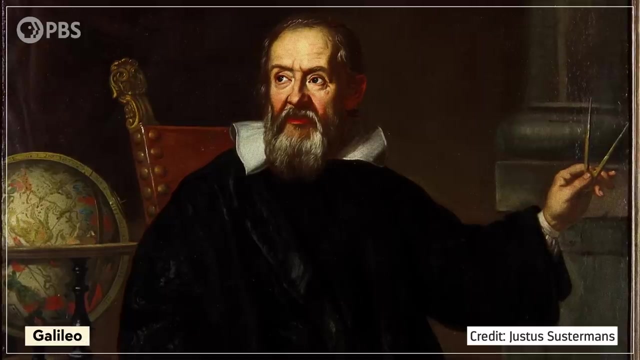 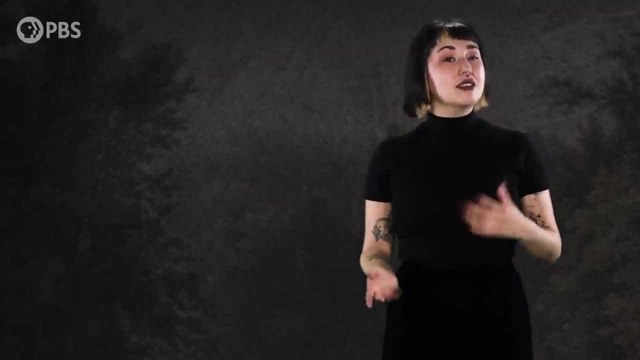 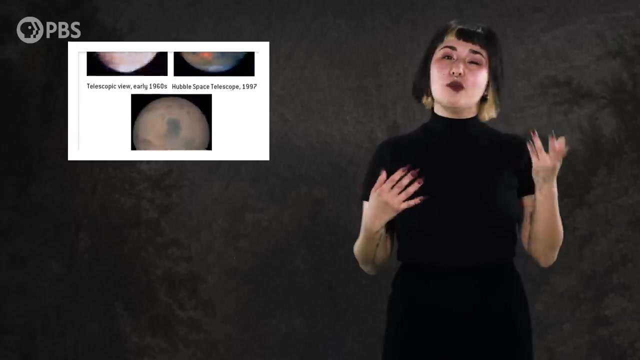 Mars has meant a lot of different things to lots of different people over human history. This strange, mobile, point of light was counted by the ancient Greeks as one of the planetes, or wanderers. And its foreboding reddish tinge meant that several ancient cultures interpreted it as a divine symbol of war, violence, and conflict. But it wasn't until Galileo first gazed at the planet through a telescope in the early 1600s that Mars started to mean something very different. As astrology gave way to astronomy, Mars was also a symbol of war, violence, and conflict. But it wasn't until Galileo first gazed at the planet through a telescope in the early 1600s that Mars started to mean something very different. As astrology gave way to astronomy, our views of Mars transformed from a mystical celestial body to an actual, physical place. 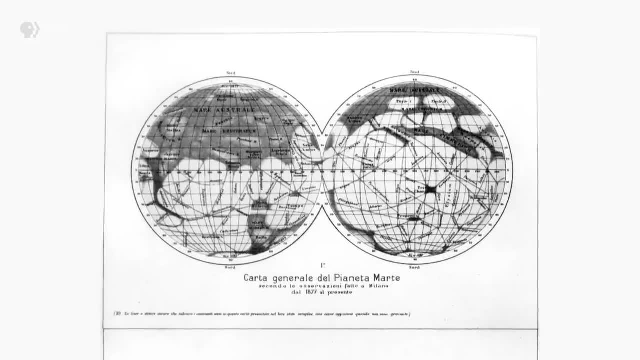 An entire other world, complete with geologic features and vast landscapes that we could observe, map out, and dream of visiting. 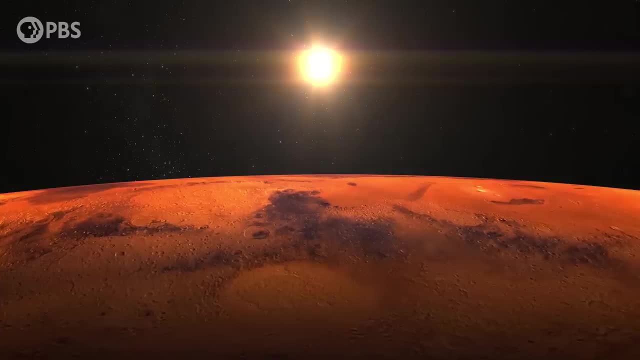 And it opened the door to another tantalizing possibility, too. As we gazed at Mars, was anything gazing back? It was a question that we could only speculate 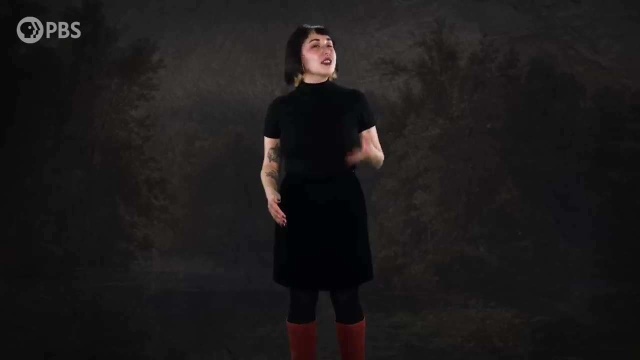 about from a distance, and boy did we, but we didn't have the technology to actually get any good answers. 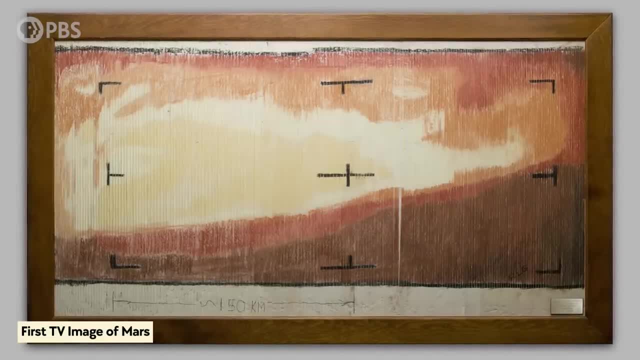 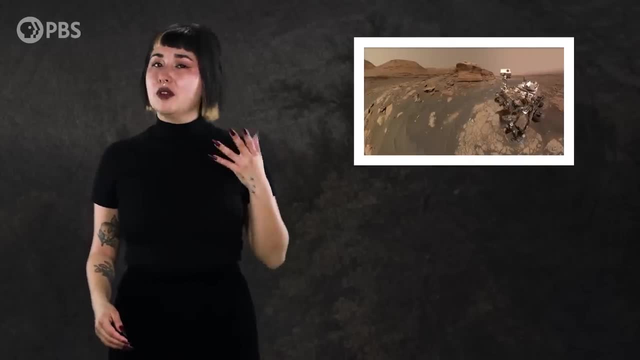 It would take until the second half of the 20th century, when our relationship with Mars transformed yet again, for us to finally investigate this possibility. Because Mars went from being a place that we could only observe from far away to a destination that we could actually travel to, or at least send machines to on our behalf. 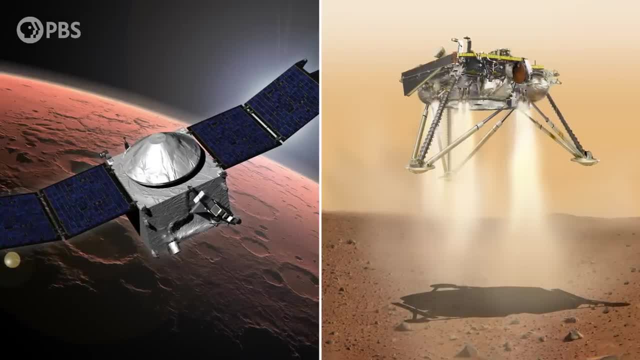 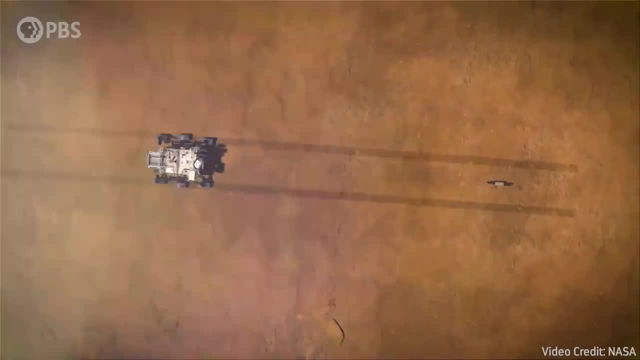 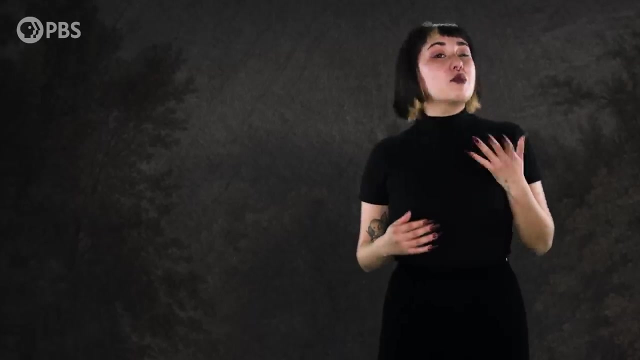 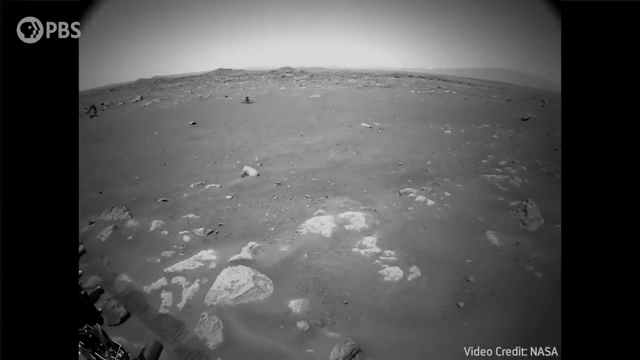 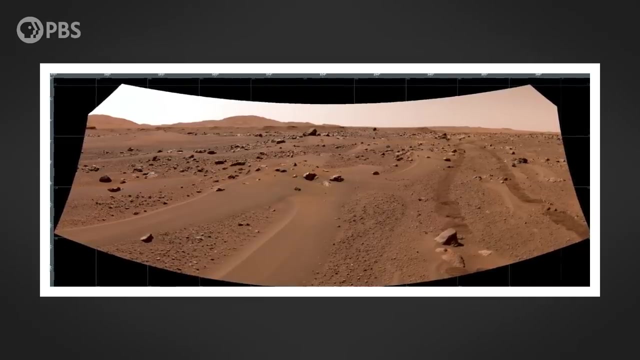 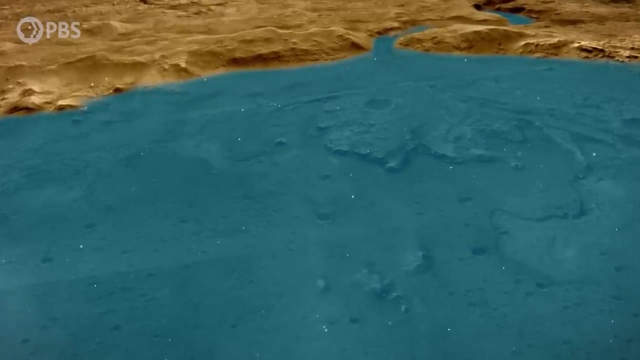 Orbiters, landers, and now rovers have revealed to us a dry, rocky, barren world with no obvious signs of life, and they've also offered us the long-sought-after opportunity to gain new insight into the natural history of the planet. Take the Perseverance rover, for example, our most recent robotic representative to arrive on the Red Planet. Since 2021, Perseverance has been working on a very important mission, to explore and study the now-dried-up lake bed of that great planet. It's looking for evidence of any ancient life that might have called that crater lake home, billions of years ago. 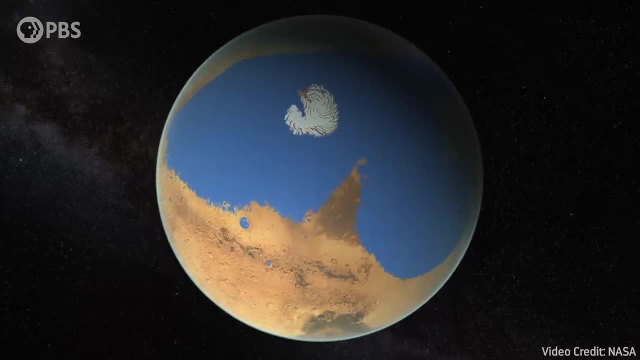 And the data that Perseverance has collected has also allowed us to trace ancient geological events from that more dynamic period of Mars' history. Like the story of that flood, nearly 4 billion years ago. 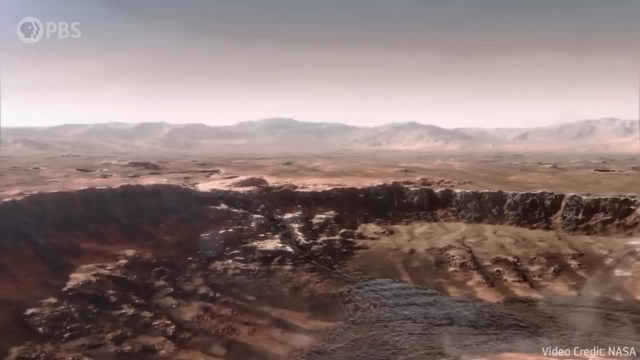 Back then, the planet had a thicker atmosphere, and was much warmer, wetter, and suitable for life. 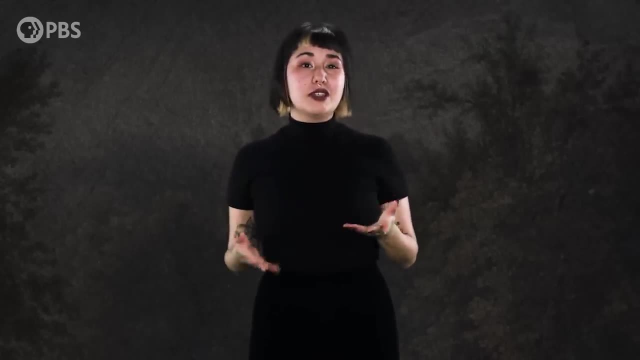 But to understand how that happened, we're going to have to find out. But to understand how that happened, we're going to have to find out. But to understand how that happened, we're going to have to find out. But to understand how and why Mars changed into what it is today, we need to go back to its formation. 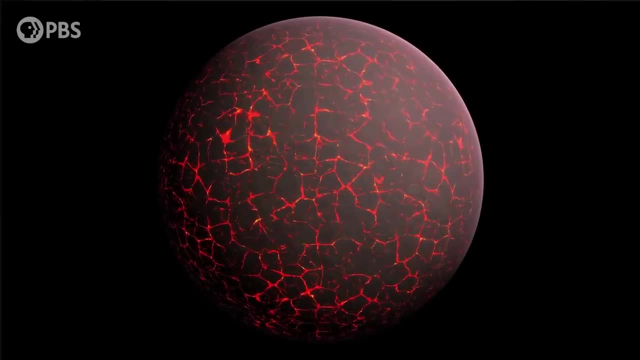 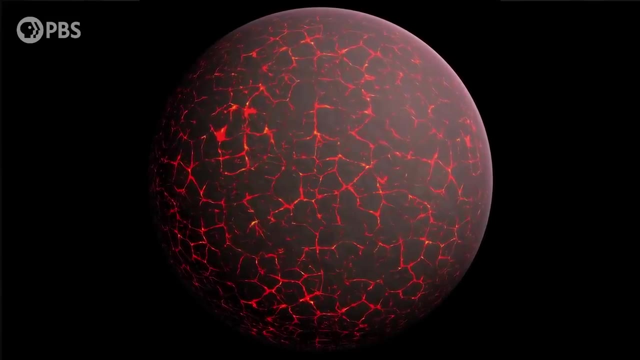 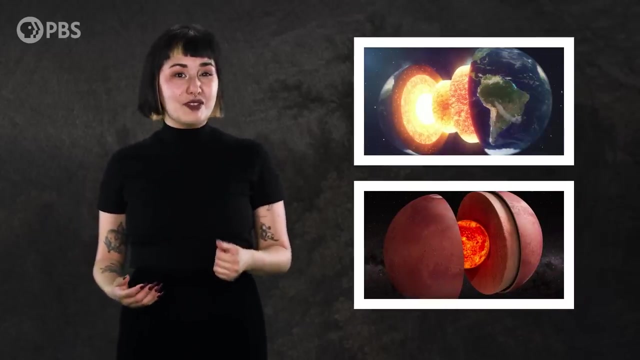 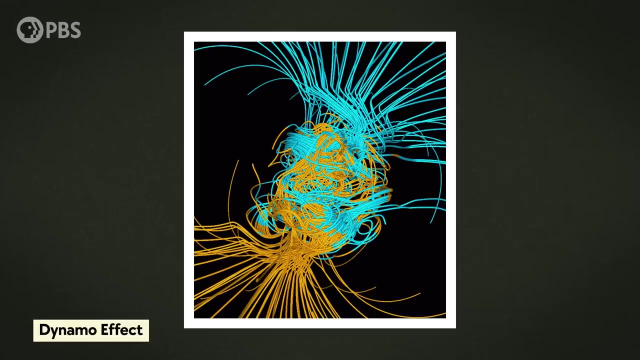 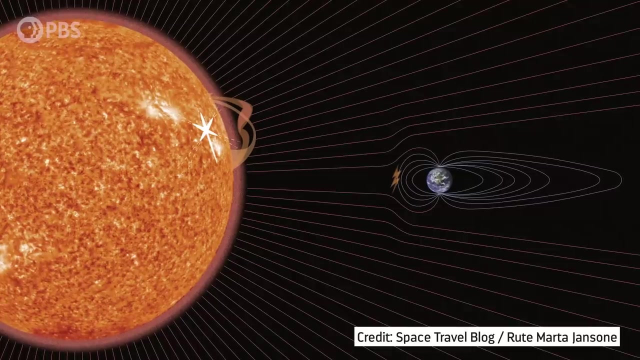 See, Mars' origin story was very similar to Earth's, with a few important differences. Both planets formed around 4.6 billion years ago from clouds of dust and rocky debris orbiting our Sun. At their centers were partially molten cores of iron that gave both planets powerful magnetic fields. This was a result of the dynamo effect, the generation of a magnetosphere by the rotating, convecting, and electrically conducting liquid iron in the outer core. Now we're lucky enough to still have an active and powerful magnetosphere here on Earth, more than 4 billion years later. 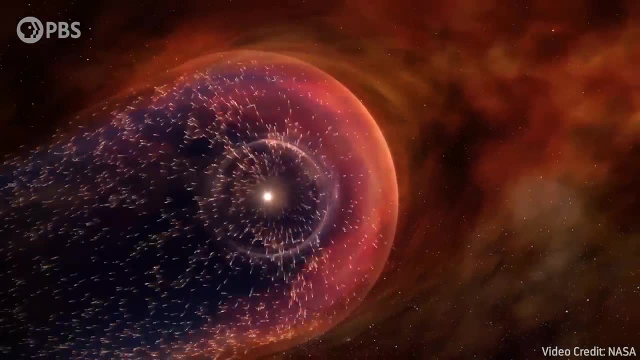 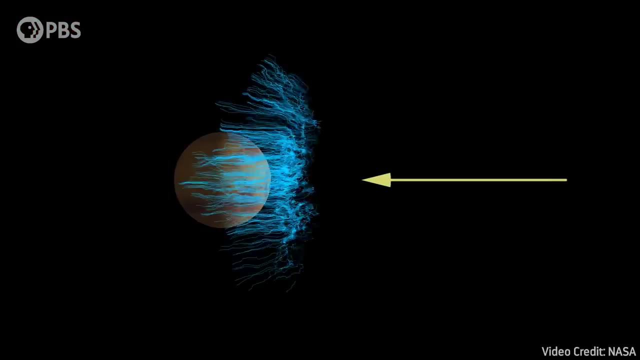 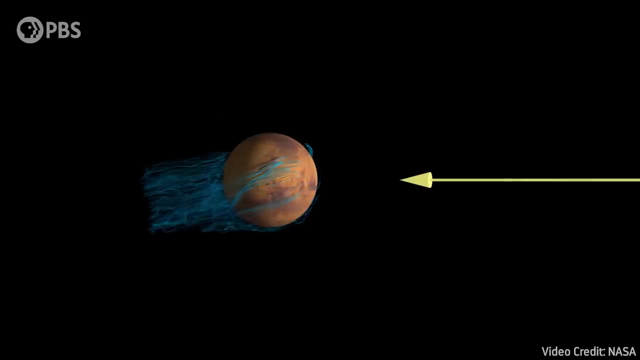 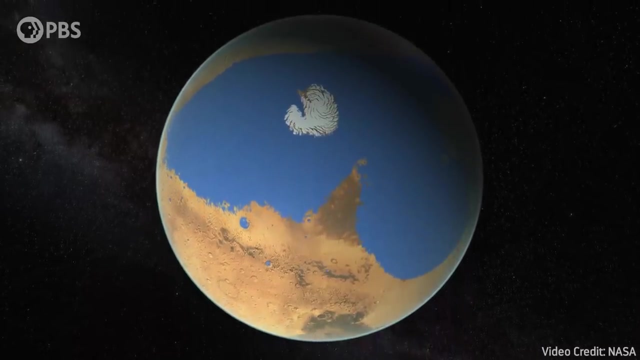 It acts as an invisible shield, protecting our atmosphere from being eroded by solar wind, charged particles belched out from the Sun. But Mars has lost its magnetosphere, and with it, protection from those solar winds. Over time, the atmosphere has changed. They stripped away its thick atmosphere, its warmth, its protection from radiation, its liquid water, and, it seems, any life it might have once had, too. Because Mars' dynamo switched off sometime after 3.7 billion years ago. We can tell, because those are the youngest Martian rocks that are still magnetized, which happens when lava cools in the presence of a magnetic field. 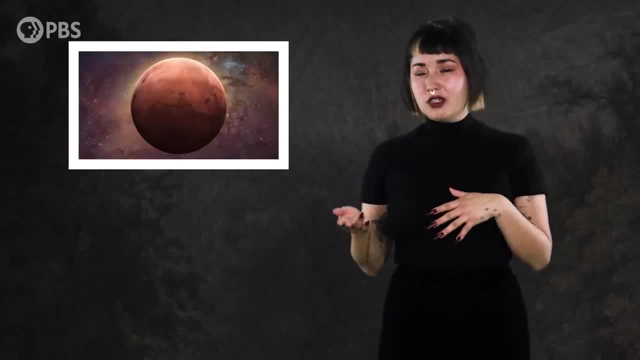 We're still figuring out exactly why its switched off, but a big part of it may have simply come down to size. 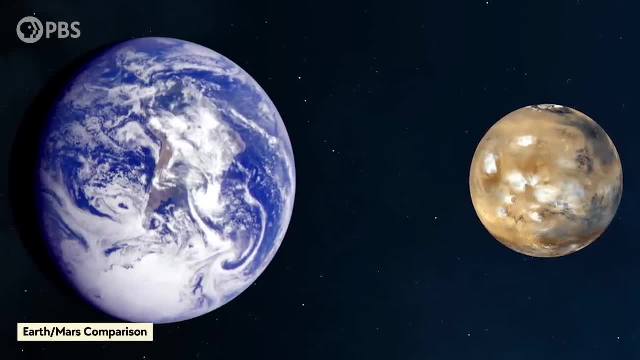 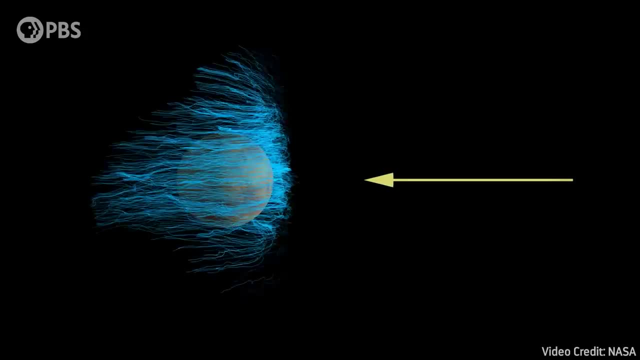 See, Mars is only around half the diameter of Earth, so its core cooled down much faster after the planets formed. This shut off the dynamo effect and exposed the atmosphere to the full force of the solar winds. 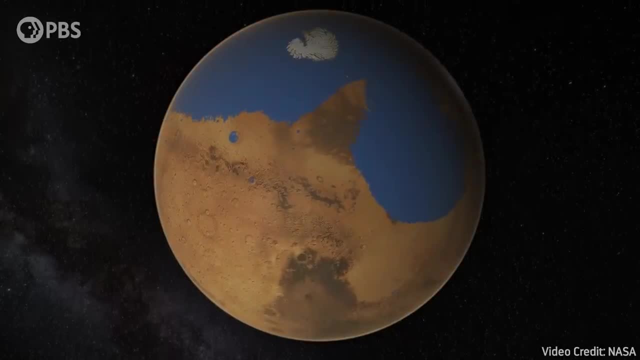 The planet's rivers, lakes, and perhaps even an ancient ocean all vanished as the water either froze, got trapped in rocks, or was lost to space without a thing to hide. But it was still there, and it's still there. It's still there, and it's still there. It's still there. 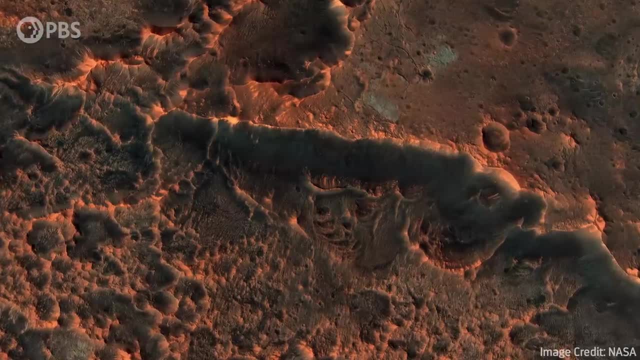 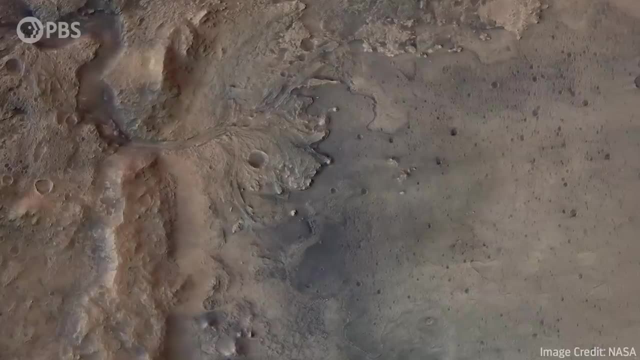 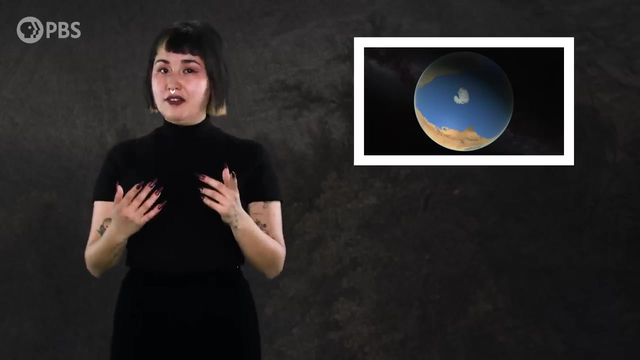 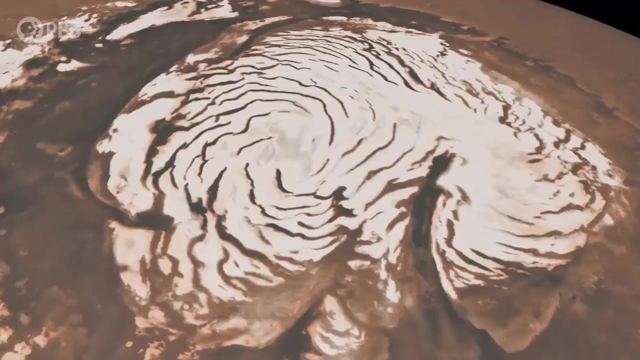 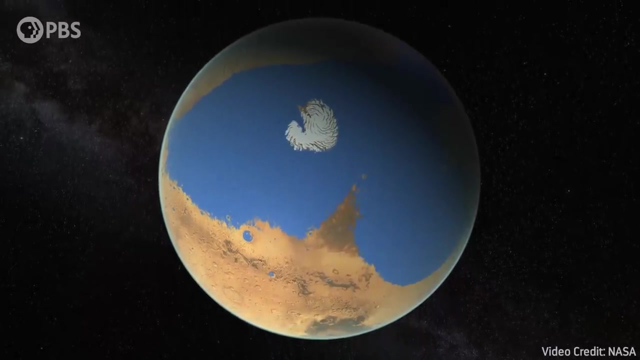 atmosphere to retain it, though they left behind the valleys, lakebeds, and shorelines that they carved into the planet's surface, prime targets in our search for past, or present, Martian life. Because the question is, if life had emerged during that long-gone age of habitability, could some especially resilient lineages have stuck around? Maybe by moving underground, or to the polar ice caps where some amount of liquid water still exists? After all, if studying life on Earth has taught us anything, it's that life, mmm, finds a way. 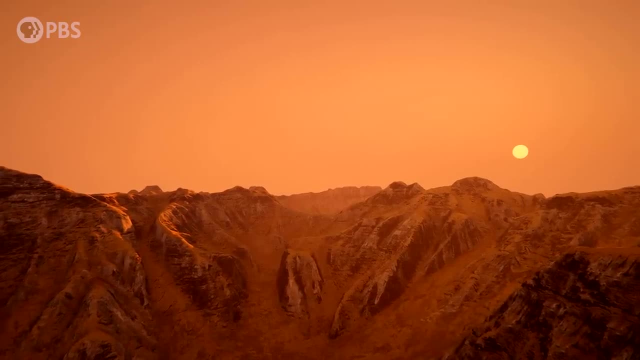 And species, especially microbes, can often adapt to thrive in even the most extreme of environments. Or, if not, could any evidence of past life have survived after all those billions of years? 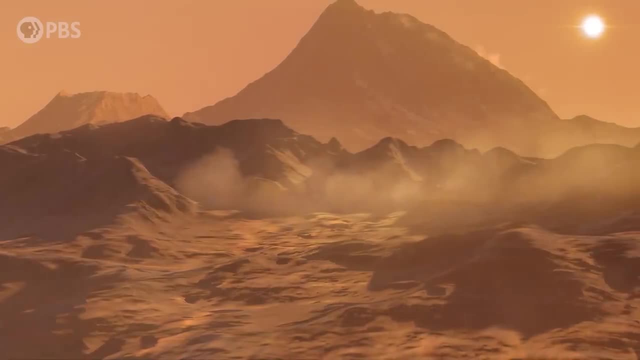 While we haven't found any evidence of past life, we do have evidence of past life. While we haven't found any evidence of past life, we do have evidence of past life. While we haven't found any definitive evidence of Martian life yet, we have found some clues. 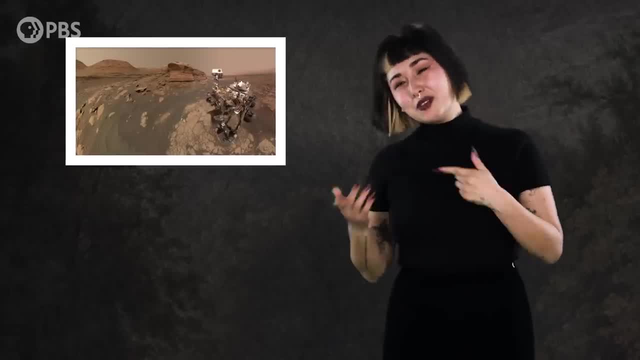 In 2018, for example, Perseverance's older sibling, Curiosity, made an intriguing discovery. 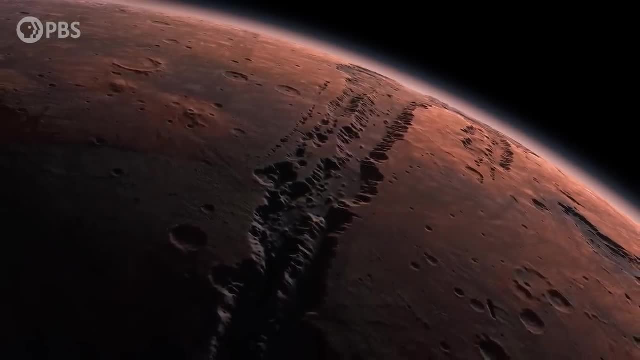 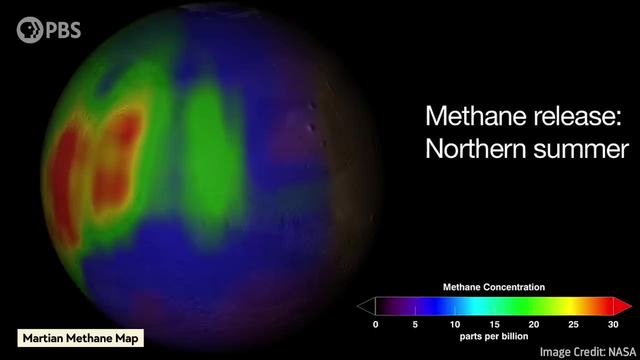 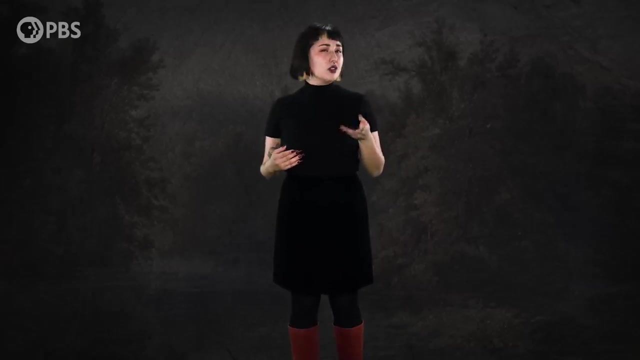 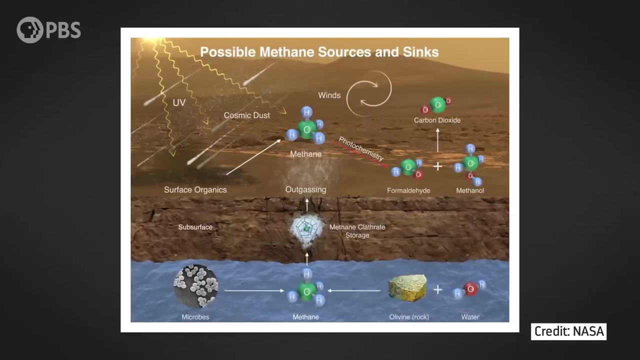 It collected data showing that the concentration of methane in Mars' thin atmosphere, a gas which on Earth is primarily produced by living organisms, seemed to cycle seasonally. This suggested that the gas might be... seeping out from underground reservoirs, which could potentially be a byproduct of microbial life below the surface where there might be liquid water and where there's better protection from radiation. Plus, both Curiosity and Perseverance have also found a variety of organic molecules in Martian rocks on the surface that are over 3 billion years old. All life that we know of is carbon-based. 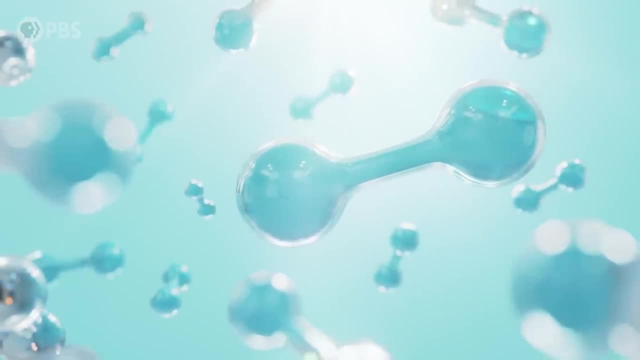 So, organic molecules are the necessary raw materials for, and potential trace of, ancient carbon-based life. Now, to be clear, neither of these discoveries means that life either definitely used to exist on Mars or still does today. Both could also just be a result of chemical and geological processes rather than biological ones. 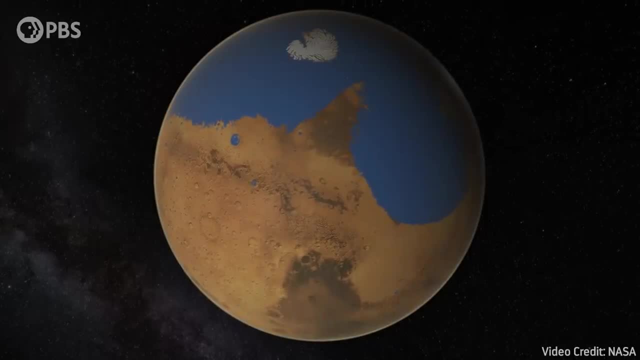 We still don't know that for sure. But there are basically three possible options. Mars never had life. It took life at some point, but it died out. 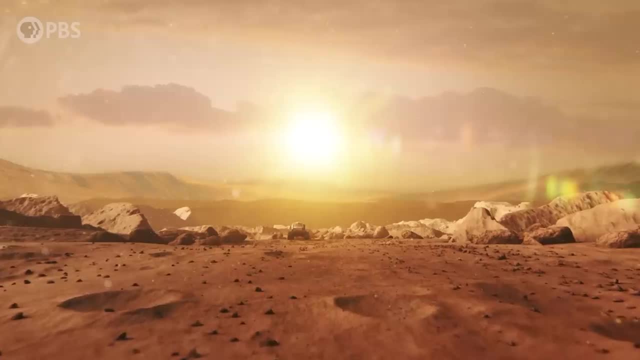 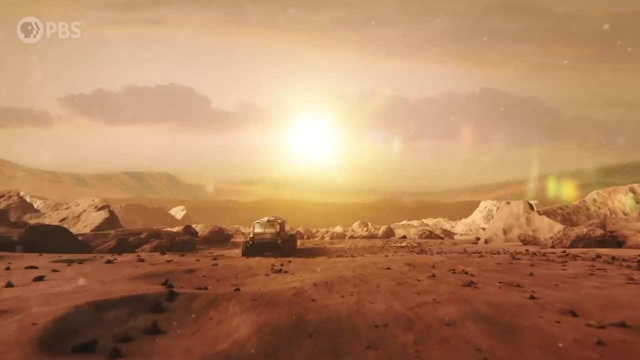 Or Mars had life and still has it today. And figuring it out might even require another transformation in our relationship with the red planet. 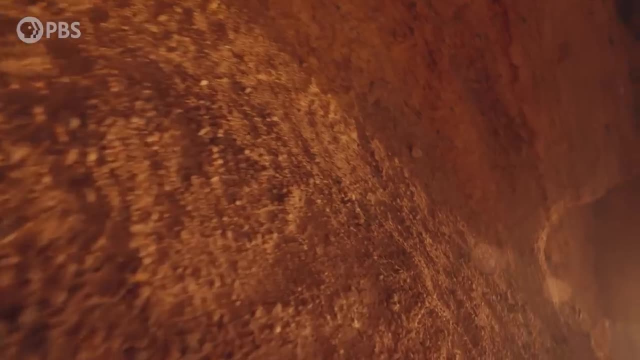 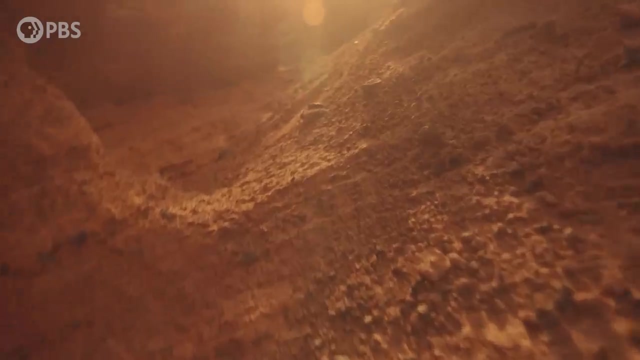 We may need to bring Mars to us. By returning some of the most promising samples to Earth, we could study them in much more detail than our rovers alone can on the planet itself. 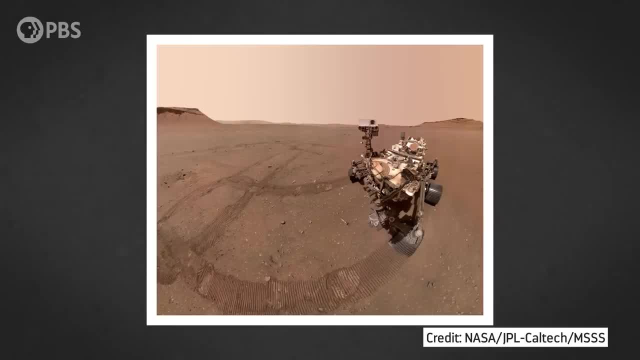 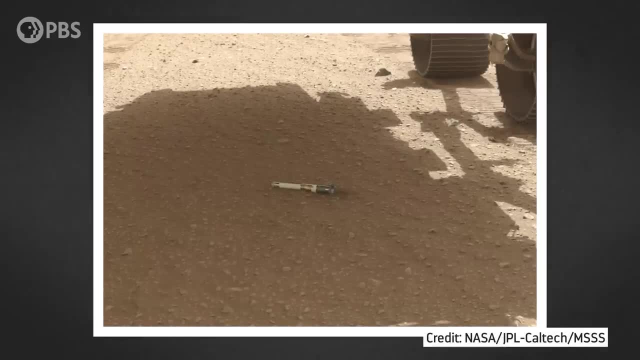 So in late 2022, Perseverance carried out one of its most important orders. It collected a rock sample from the crater, packaged it in a titanium tube, and left it at an assigned spot nearby. 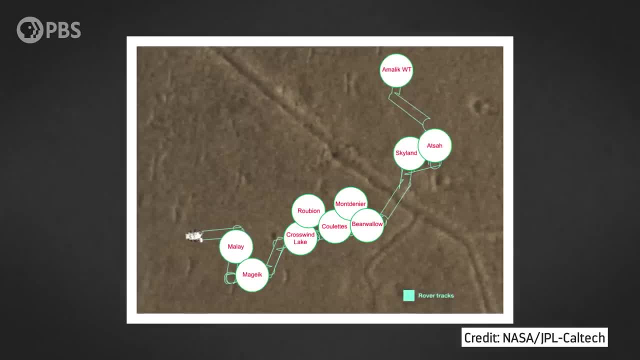 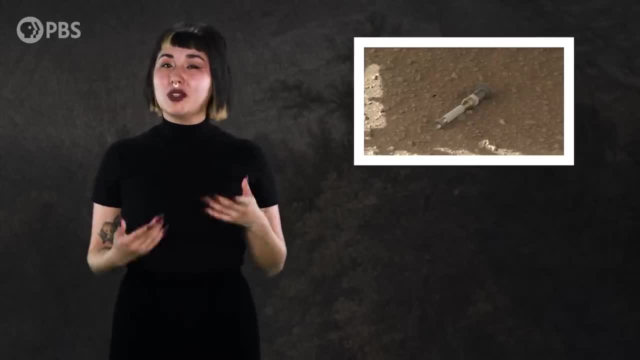 This was the first of many samples of rock, sediment, and atmosphere that Perseverance has been tasked with carefully collecting. And in the early 2030s, a robotic mission will arrive, retrieve some of the samples, and return them to Earth for analysis. 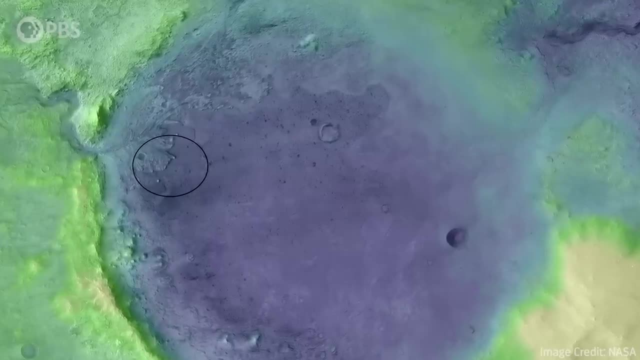 Scientists hope that studying actual samples of Mars in our labs from that ancient core, will help us find out more. 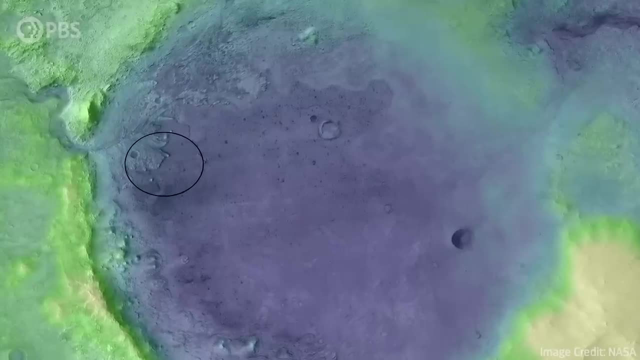 We are excited to find out more about this new science. Once we do that, we will have the chance to study tons of different effects and can create indelible records last year. 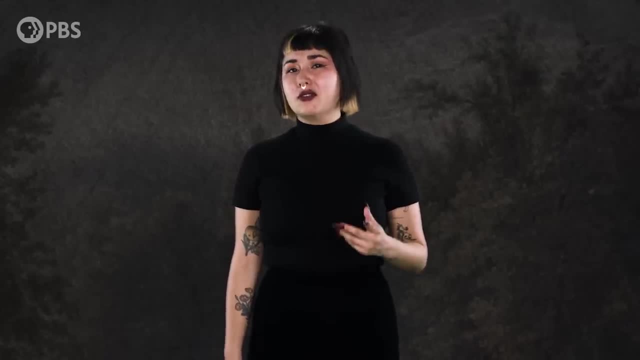 Whatever the answer is, it will radically change how we understand the nature of life itself. 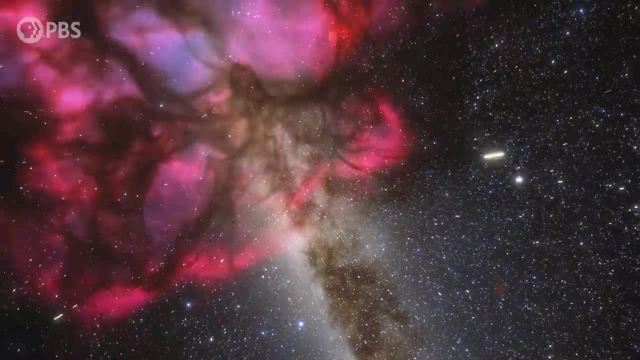 Is biology common or rare in the universe? Is life on Mars related to life on Earth?